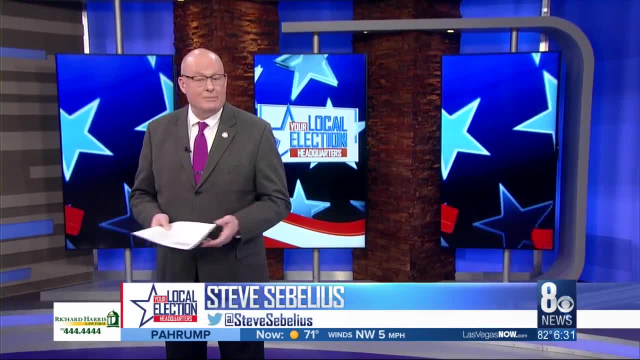 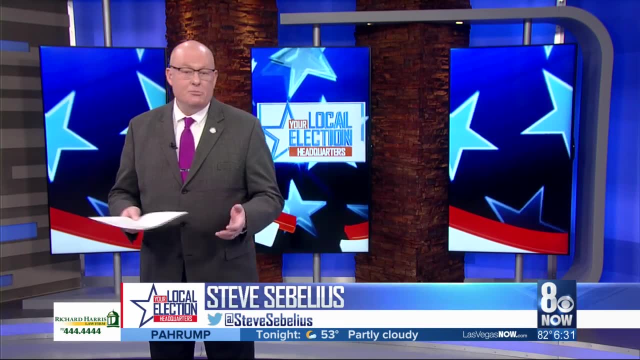 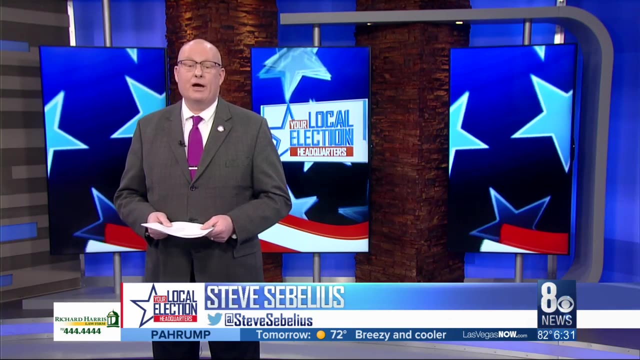 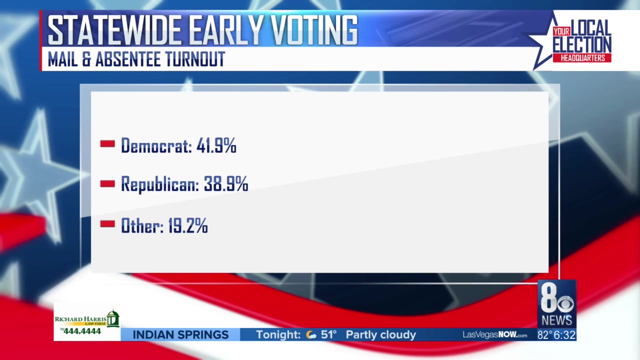 voters. but you wouldn't know that from looking at the early voting mail and absentee ballots, Republicans and Democrats are nearly even in statewide voting, and in one key county in the state, As of this morning, just 11,196 more Democrats than Republicans had cast an early vote, And that means those statewide races are probably going to be very close. Overall, Democrats account for 41.9% of all early votes, with Republicans just two points down at 38.9%, According to the Secretary of 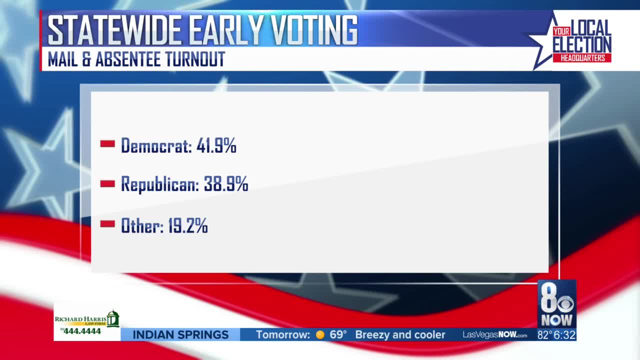 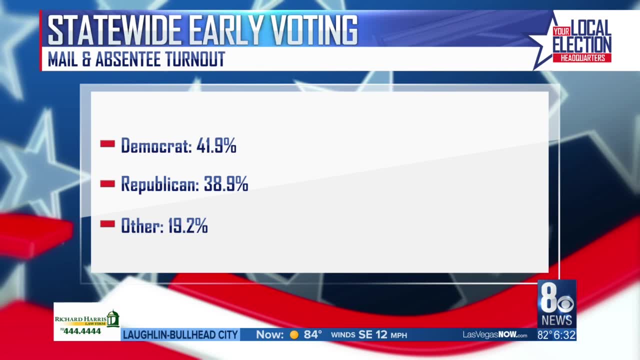 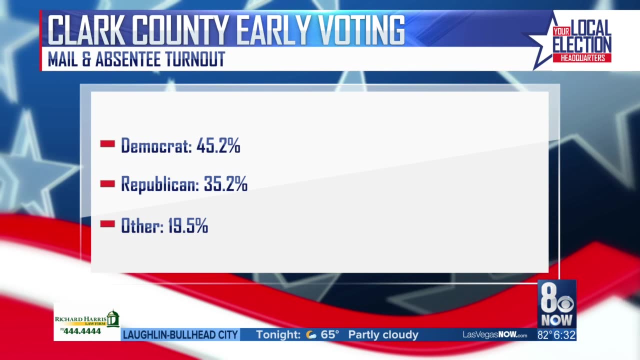 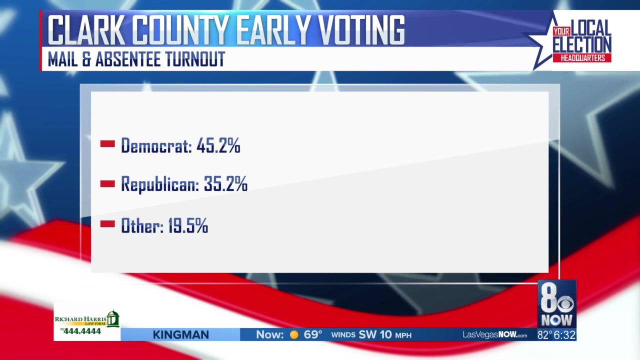 State. nonpartisans and minor party ballots account for the remaining 19.2% of ballots. Both Democrats and Republicans are performing better than their respective party registrations, with Republicans turning out at a slightly higher percentage than their Democratic counterparts. Here in Clark County, where most Democrats reside, Democrats are doing a little better: 45% of all ballots cast belong to them, with 35% for the Republicans. The remaining 19.5, those are nonpartisan voters. The Democratic advantage down here is: 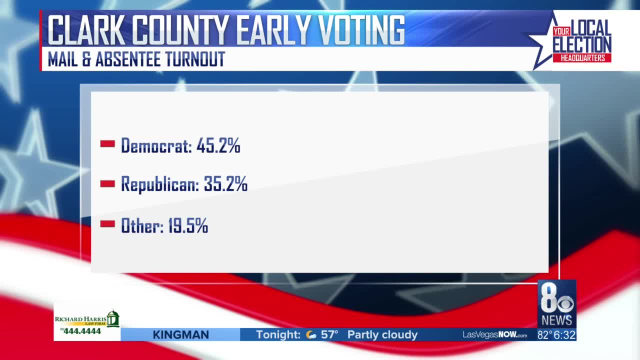 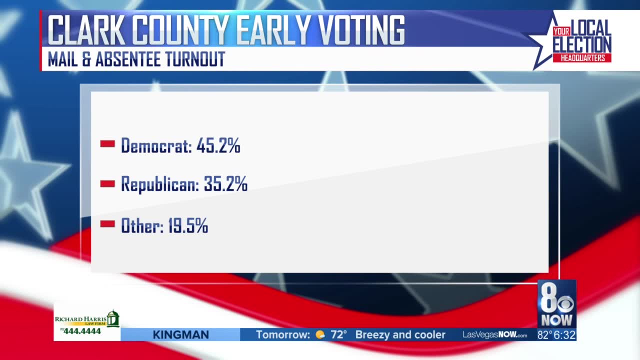 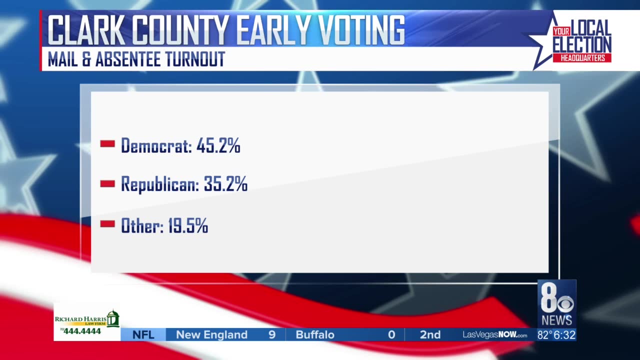 more than 25,000 voters as of today. But up in the critical swing county of Washoe things are very close. Democrats cast 41.7 percent of early in-mail ballots, while Republicans cast 40 percent. Nonpartisan and minor party voters account for 18.3 percent up in Washoe. That's critical. 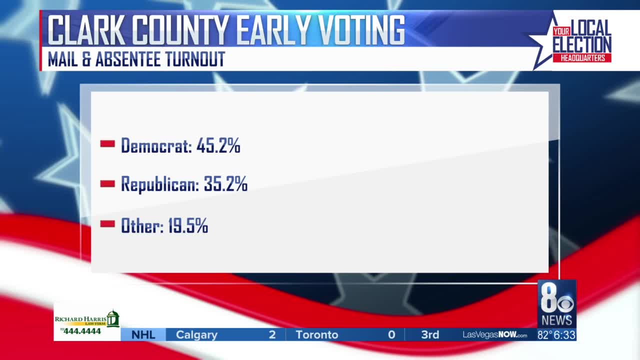 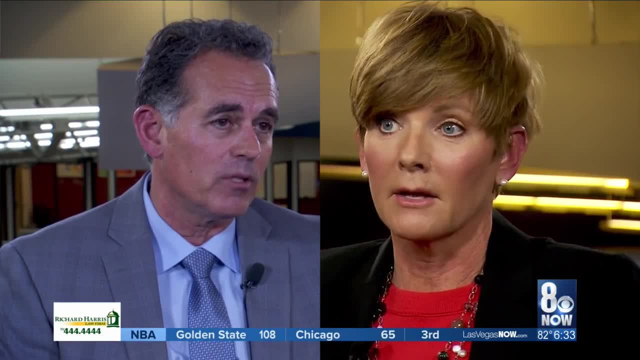 especially to Democrats running statewide. About 1,100 more Democrats have voted in Washoe than Republicans. Now, looking at some of the big races, Democrats barely lead Republicans in Congressional District 3, where Republican Danny Tarkinian is facing off with Democrat. 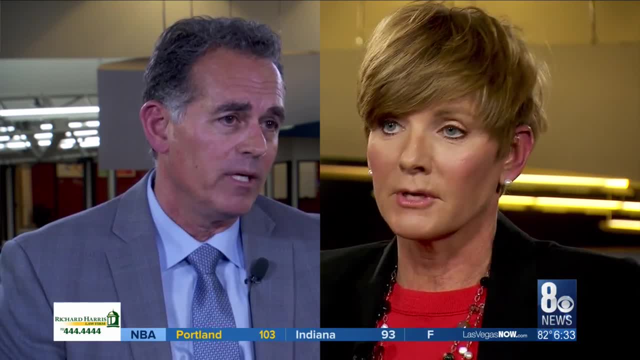 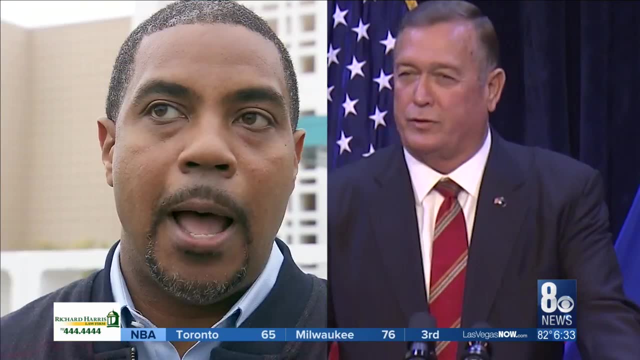 Susie Lee, Democrats are about two percentage points ahead, but in real numbers they're only 2,100 voters up. That doesn't count any of the 20 percent of ballots cast by nonpartisans In the 4th Congressional District, where Democrat Stephen Horsford is facing Republican. 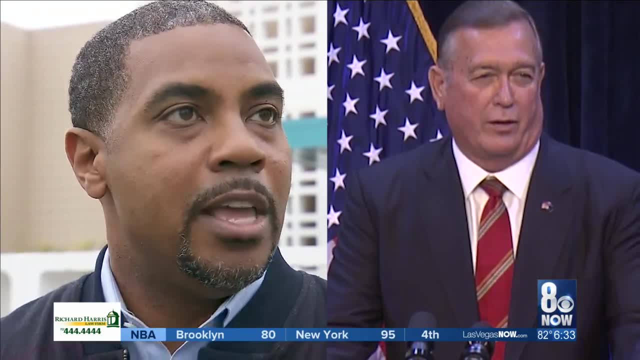 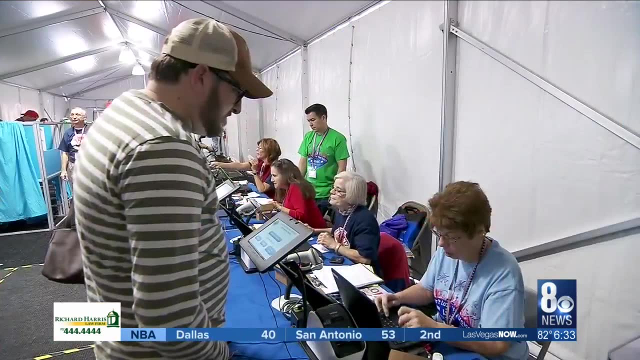 Cresson Hardy Democrats have a slightly larger margin: 11 percentage points works out to about 9,000 actual votes. And in the key State Senate, District 8,. the battle- battle between Republicans and Democrats- is about to begin Between former Assemblywoman Marilyn Dondero-Loop, the Democrat, and Valerie Weber, the Republican.